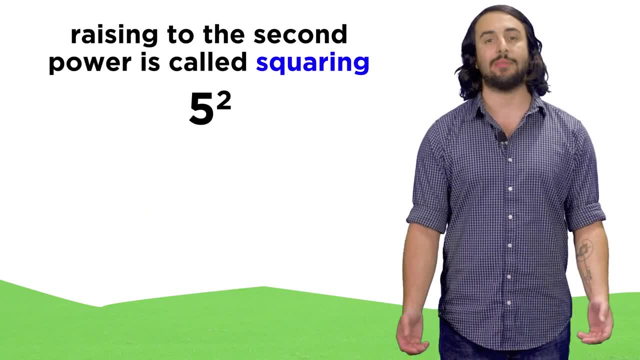 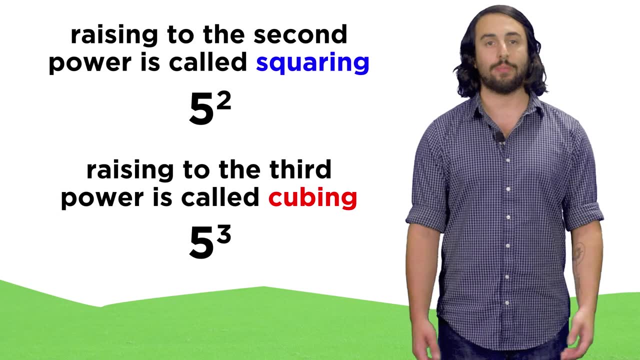 two times two. When we raise something to the second power, we are squaring that number, So we can say five squared. When we raise something to the third power, we are cubing that number, So we could say five cubed. 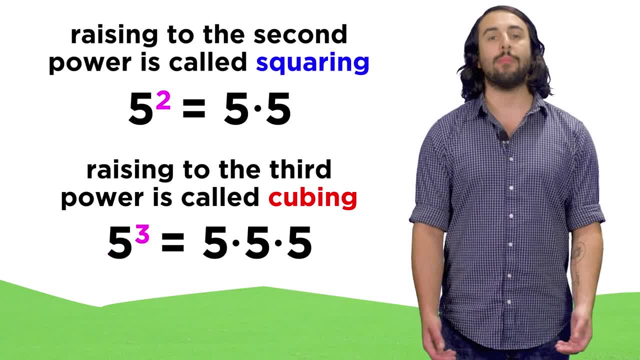 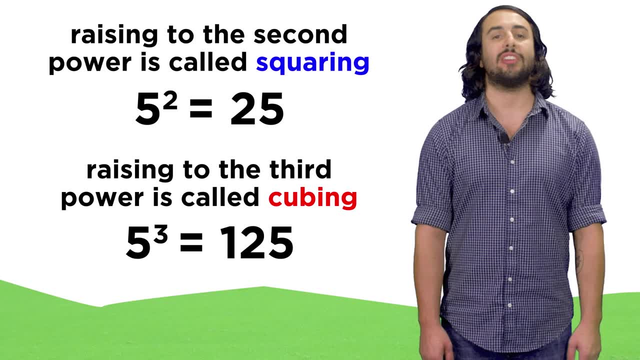 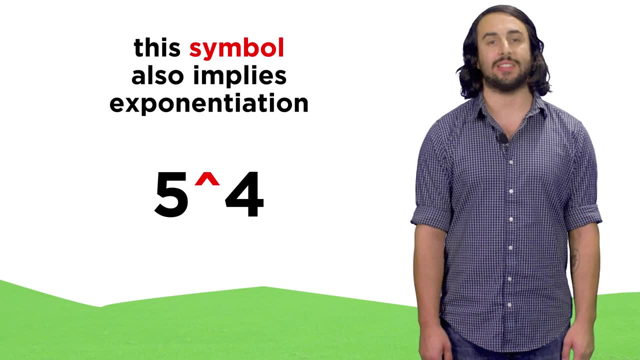 In each case we can write down the base number, the number of times indicated by the exponent, and do the multiplication, which gives us twenty-five and one hundred twenty-five respectively. Sometimes, instead of the superscript, we might see this little hat symbol here and when. 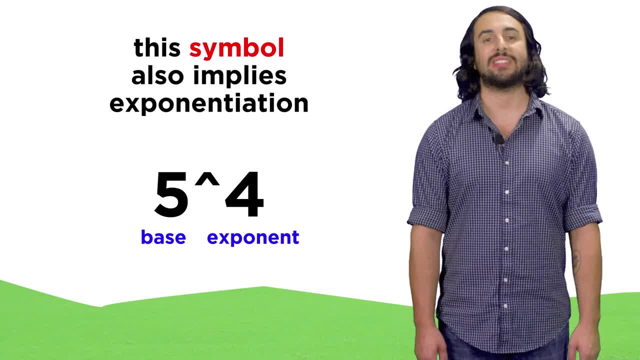 we see this: the first number is the exponent and the second number is the exponent. So we can write down the exponent and do the multiplication, which gives us twenty-five and one hundred twenty-five respectively. The first number is the base and the second number is the exponent. so this is five to 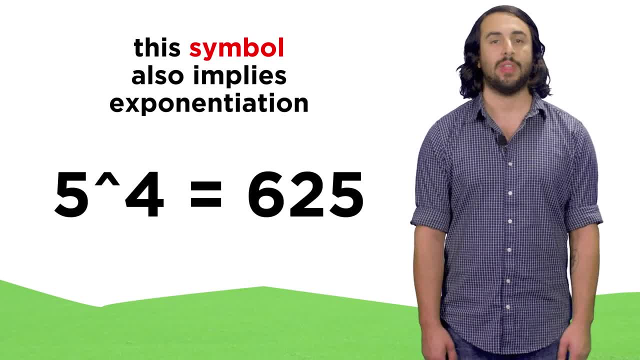 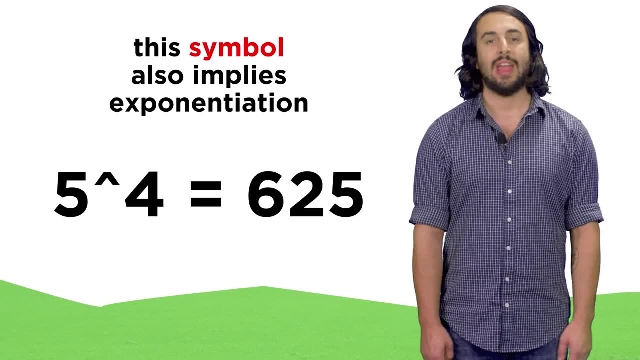 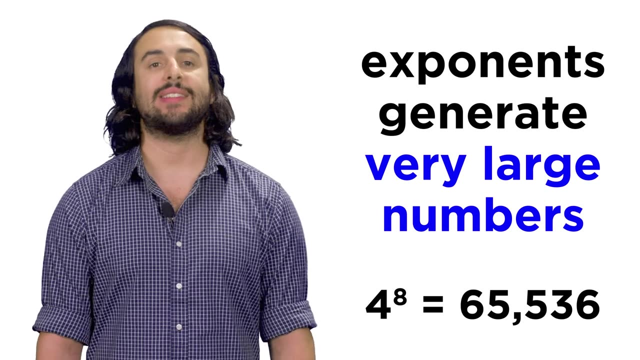 the fourth power or six hundred twenty-five. This is typically used when someone has written the expression without access to the superscript function, and this symbol is needed to imply exponentiation. One thing we will notice immediately is that with exponents, numbers get very big, very. 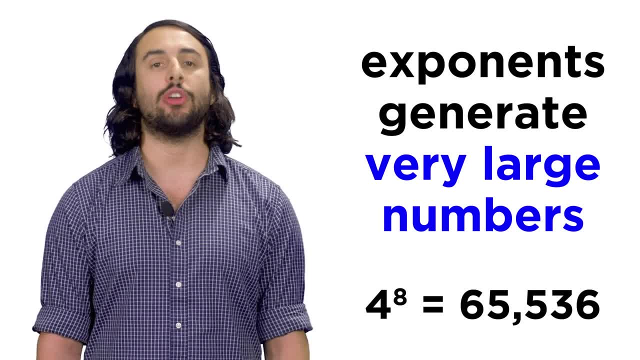 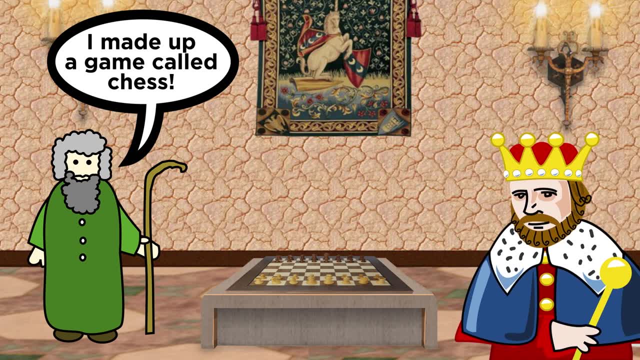 fast To see exactly how big. let's examine a number. Let's examine an old Indian legend which goes like this: A wise man invented the game of chess, which the king immediately adored. He liked it so much that he offered the wise man any reward of his choosing. 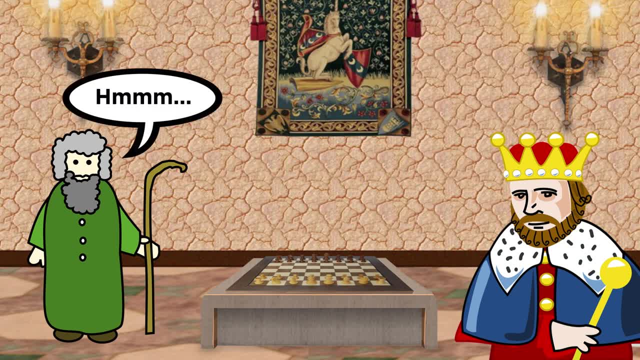 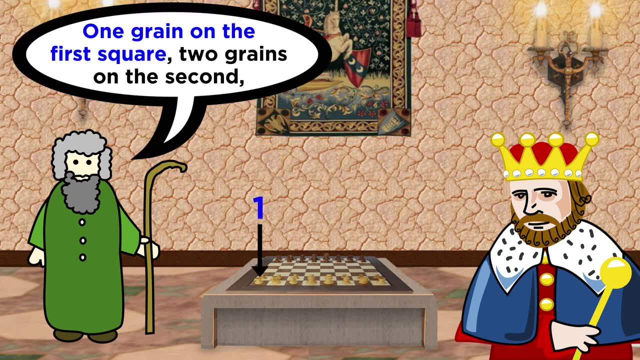 Being a shrewd mathematician. his request went as follows. He said: I am a modest man. I desire but a few grains of rice. Take this chessboard and place one grain of rice on the first square, then two grains on the second. 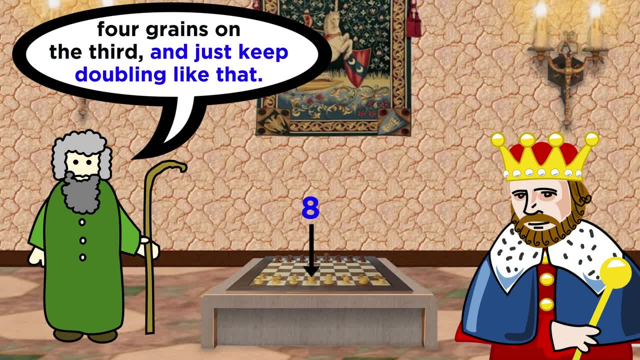 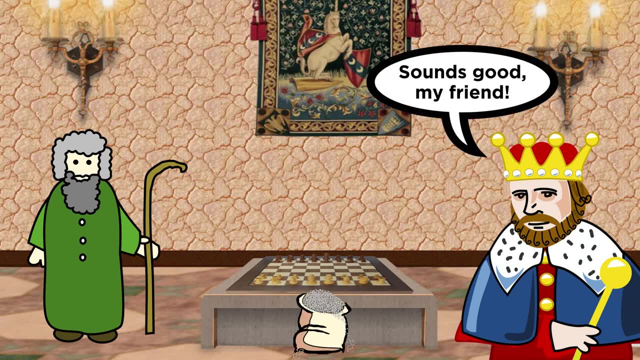 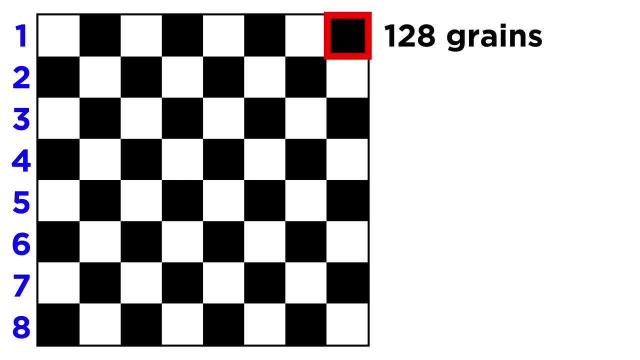 And then four grains on the third. Continue in this manner, always doubling the previous number, until all the squares are full. The king began to oblige, but he very quickly found how impossible this request was to fulfill. By the end of the first row he was already up to a hundred and twenty-eight grains. 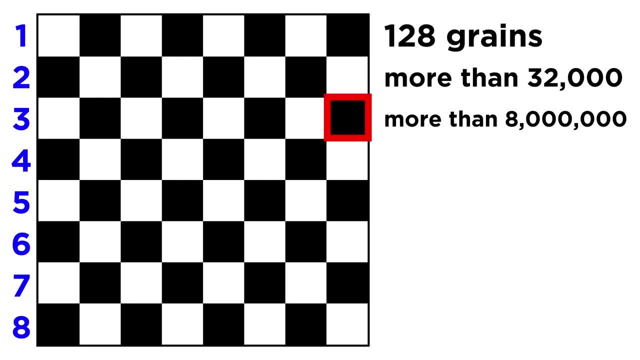 By the end of the second row, over thirty-two thousand, The third more than eight million, The fourth over two million, The fifth over two billion grains of rice. And that's just half the board. On the final square, the king would have to place over a quintillion grains of rice, which 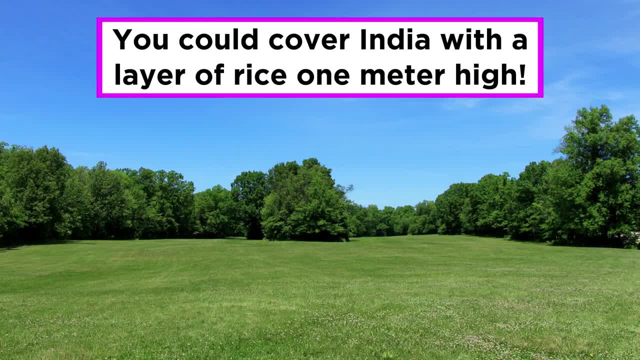 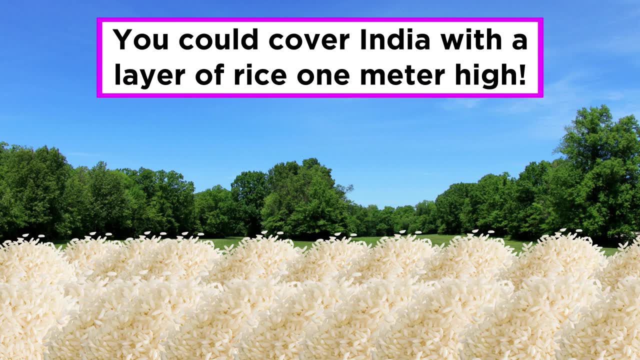 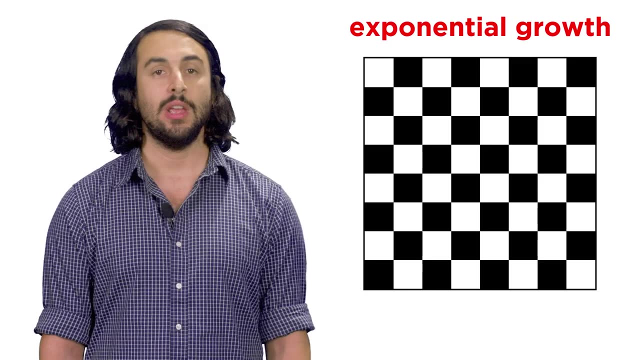 is a one, followed by eighteen zeros. That's enough rice to cover the entire country of India, with a layer of rice a meter high, and this much rice could not exist in the entire world. Luckily for the king, the wise man allowed him to pay in installments. 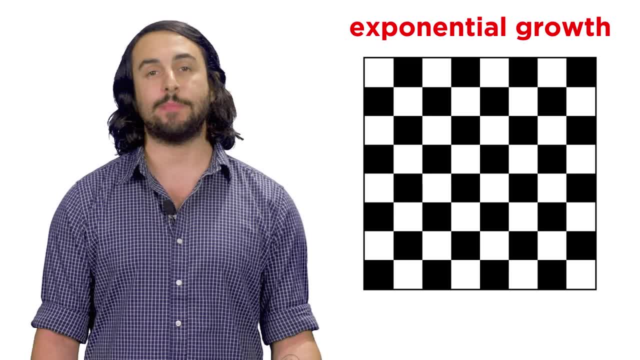 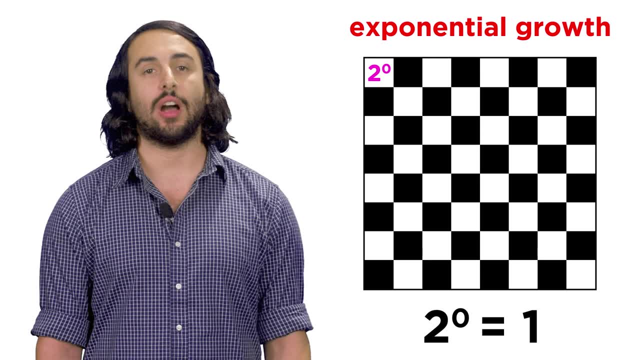 Here's a sample of exponential growth. To find the number of grains that must be placed on each square, we simply raise two to a particular exponent. We start with one, which we could think of as two to the zero, with power since anything. 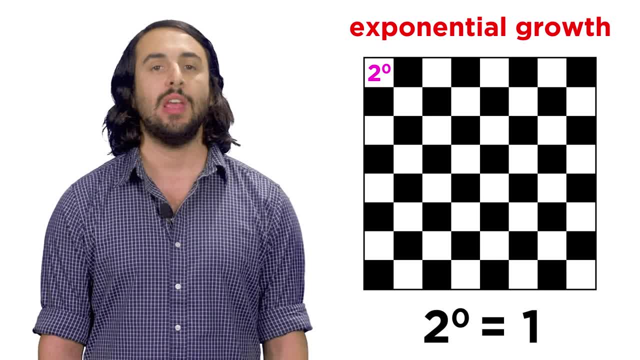 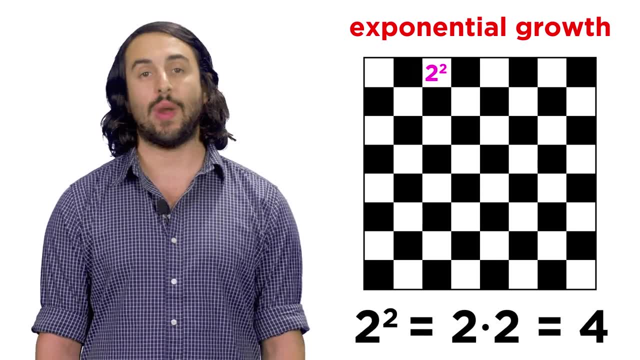 raised to an exponent of zero will be equal to one. Later in this clip we will see why this is the case. Then two to the one, or simply two, Two squared, which is two times two or four. Then two cubed, or two times two times two. 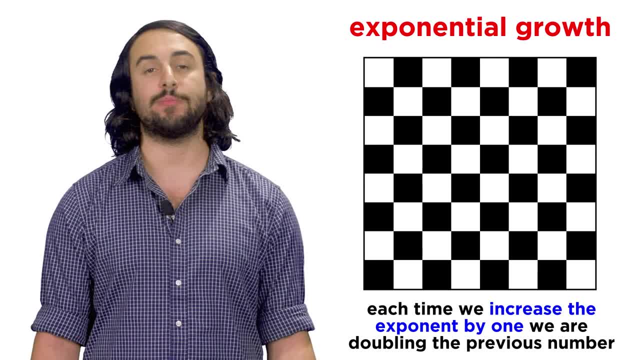 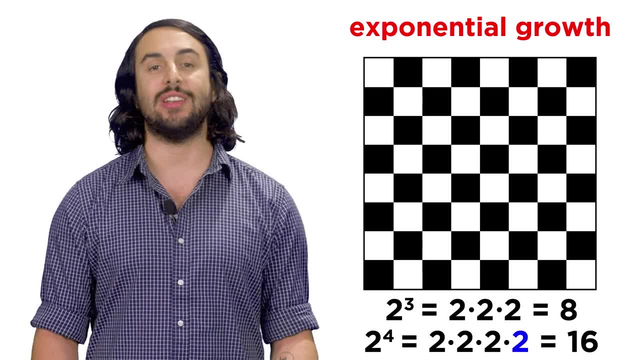 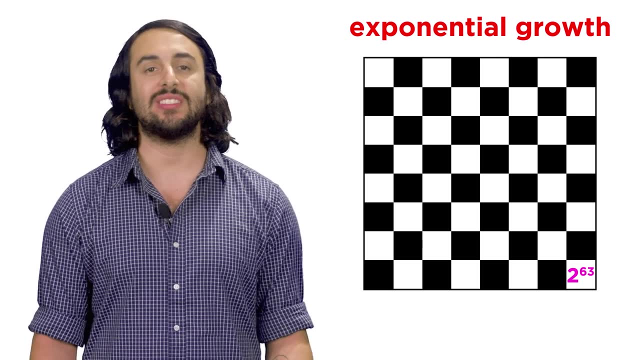 Each time we increase the exponent by one, we are doubling the previous number, because we are multiplying by two, exactly one additional time. This continues until we get to the final square, which is two raised to the sixty-third power. So we can quickly see the immense power of exponents. 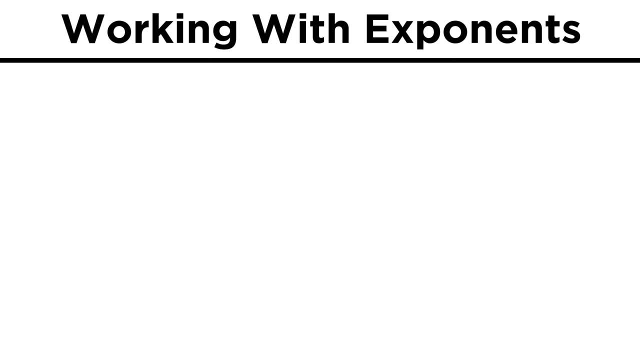 Let's try a few examples to practice. What is three to the fourth power? That would be three times three times three times three, or eighty-one. What about six to the fifth power? Well, that will give us five sixes to multiply, which equals seven thousand seven hundred. 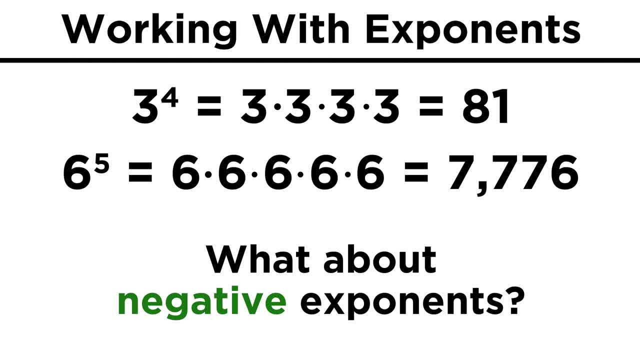 and seventy-six. Can we raise something to a negative exponent or only positive? We can do either, in fact, and when raising to a negative exponent, we simply invert the term and make the exponent positive. So the derivative of a negative exponent is one over two squared, or one-fourth. 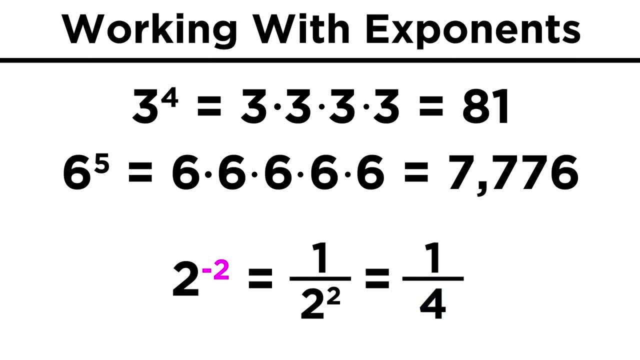 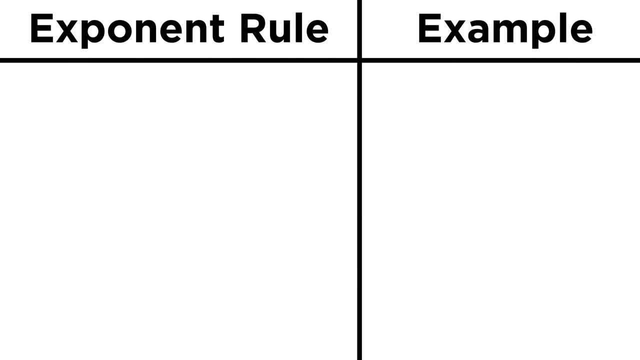 Since two squared is four, and four and one-fourth are the inverse of one another. this demonstrates precisely what negative exponents do. Another way to understand this is to learn the rules of manipulating terms raised to exponents X to the A times X to the B is equal to X to the A plus B. This must be true because 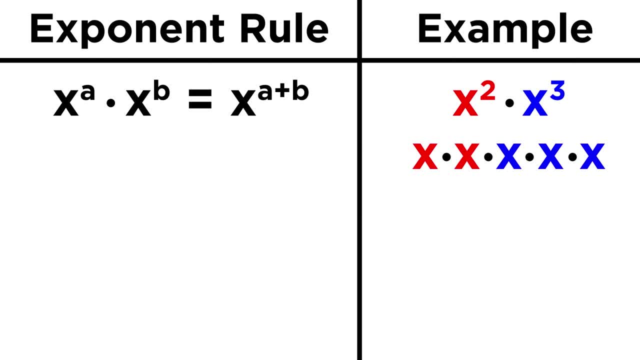 x squared times x cubed. That could be written as two x's times three x's, But that's now just five x's in a row, so we should be able to call this x to the fifth, And that's why we do a plus b, because two plus three is five and that represents the total number. 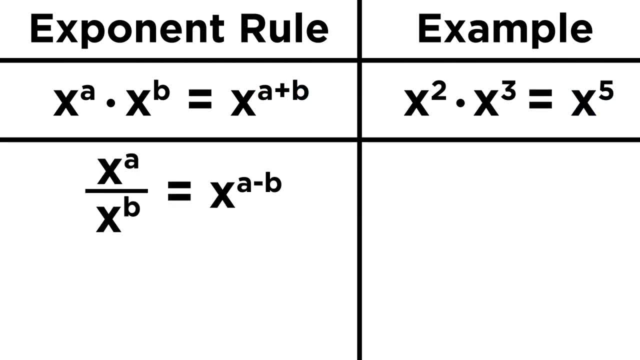 of times we are multiplying x. For division it's the opposite: X to the a over x to the b equals x to the a minus b. Again, this makes sense if we do something like x to the fifth divided by x to the third. If we change this into five x's over three x's, we can: 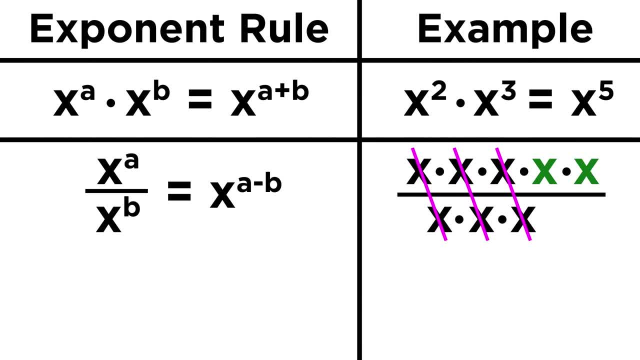 see that three of the x's cancel, leaving just two on the top, or x squared. The number of x's left is the number of them that are on the top minus the number of them that are on the bottom. hence x to the a minus b. 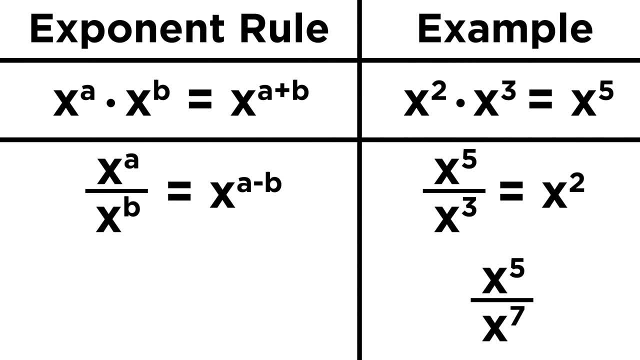 This also explains how we can multiply x to the a minus b. Now let's look at how negative exponents work. If we have x to the fifth over x to the seventh, five x's cancel and we have one over x squared, But five minus seven is. 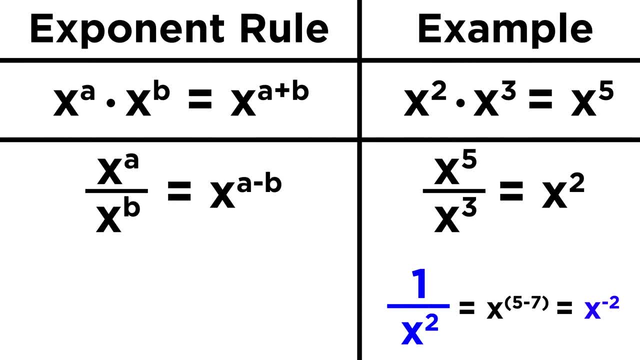 negative two. so this must be equal to x to the negative two as well. This rule also tells us why anything raised to the zero power must be one. X cubed over x cubed is x to the three minus three or zero. But it is also the case that all the x's cancel, leaving us with 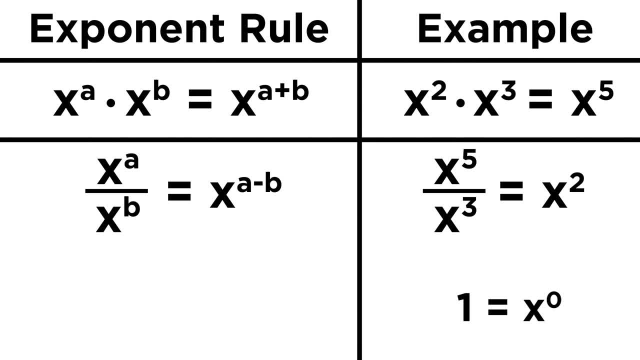 one. So anything to the zero power must be equal to one. Lastly, if we do x to the a power which is then raised to the b power, we get x to the a times b. Let's say we have x to the fourth to the second. That means we have four x's. 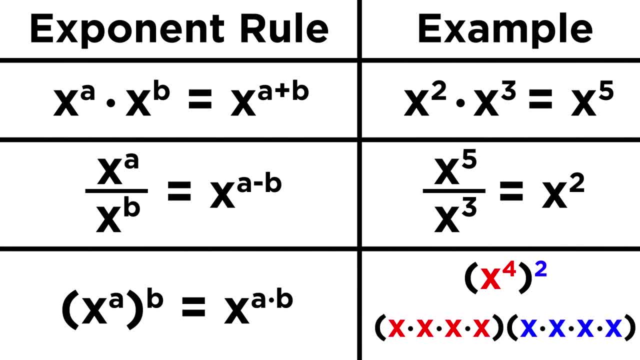 and then that whole thing is squared, meaning two sets of four x's, That's eight x's total, or x to the eighth, which is four times two. So these expressions summarize the rules for manipulating terms that are really negative, raised to exponents.